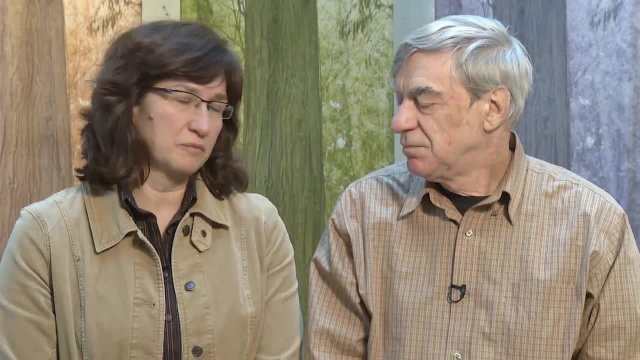 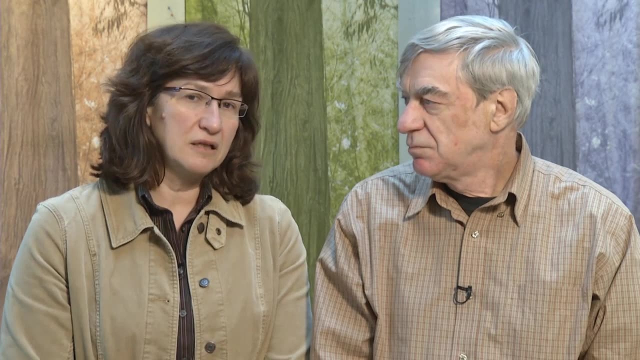 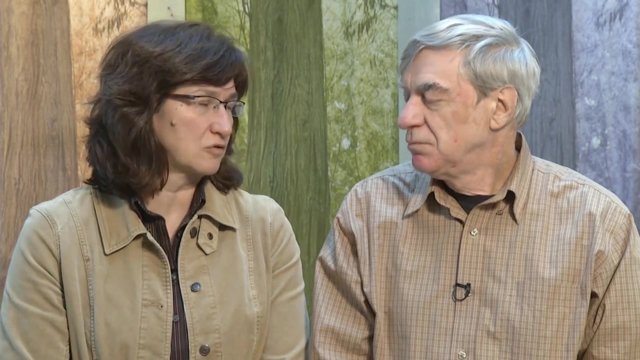 of British Columbia and now they are at the University of British Columbia, but then it spread to other BC universities like Thomson Rivers University and University of Northern BC, And lately other scientists from other Canadian universities also joined in. So at the moment this is a true Canadian collaboration in order to promote soil. 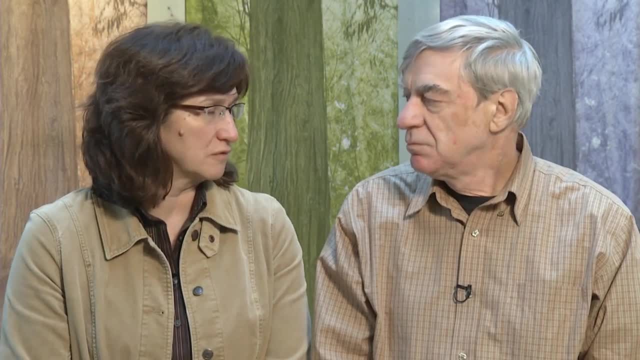 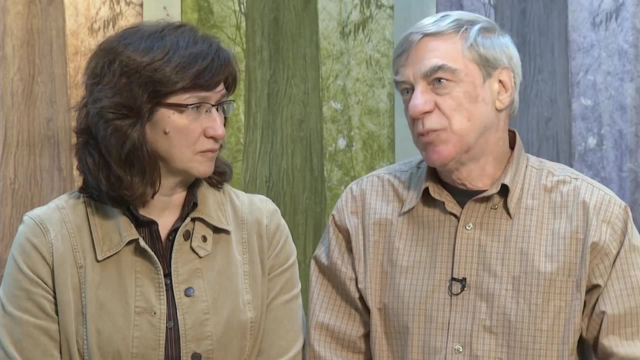 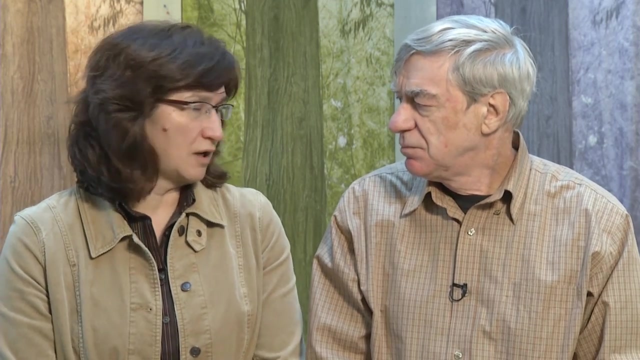 science and to teach soil science in a different or innovative way. So that explains something about how we got to where we are here. but why is this important? Well, as you know, we soil scientists are not that great in promoting our discipline beyond the 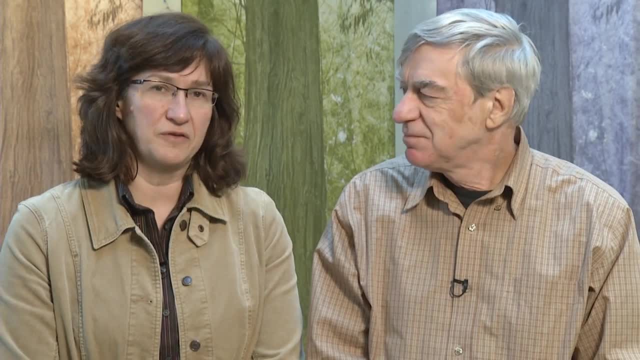 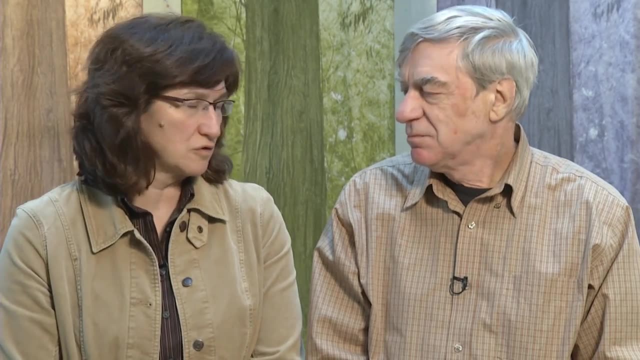 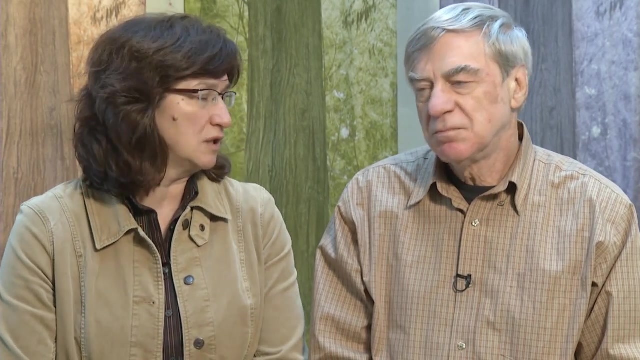 university And several of us felt that we need something different to reach a broader audience, beyond our typical university, And that's why we're here today. So we're here today to talk about soil science, And one way we thought we might be able to do this is to engage into video and multimedia and produce 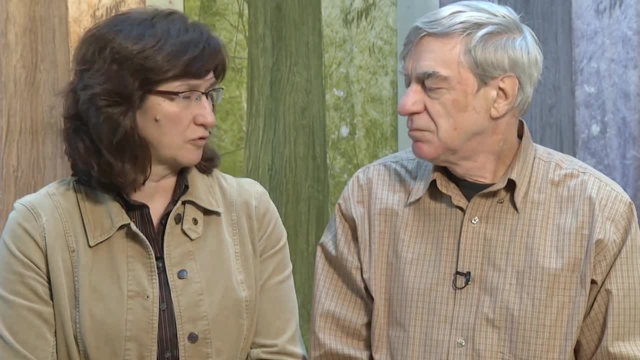 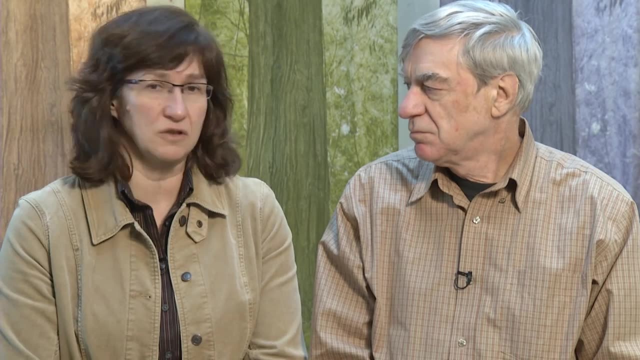 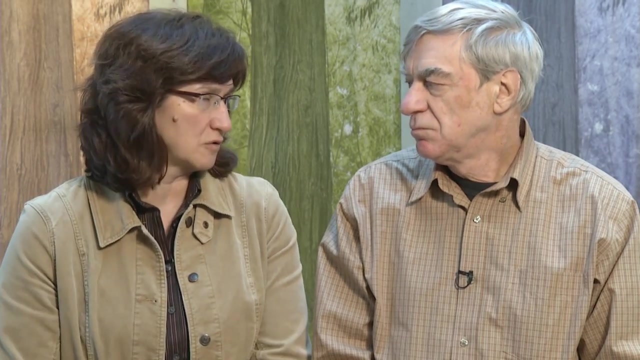 different types of resources that are not just useful for our students, but also for a broader audience, Because, as we, as soil scientists know, soil science is an extremely important natural resource which is incorporated in many aspects of our lives, and also current. issues like climate change- So soil science is an extremely important natural resource which is incorporated in many aspects of our lives- and also current issues like climate change. So soil science is an extremely important natural resource which is incorporated in many aspects of our lives- and also current issues like climate change. 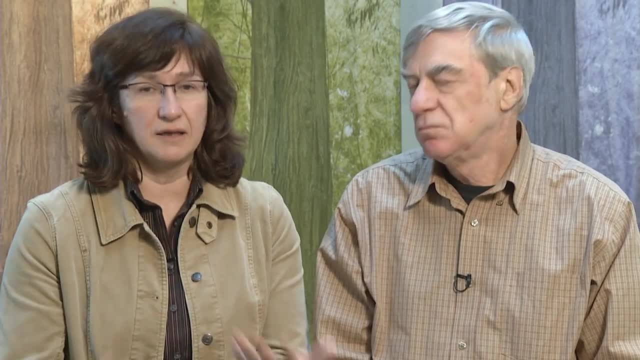 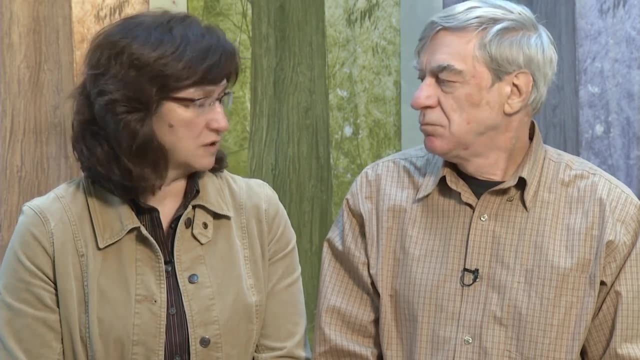 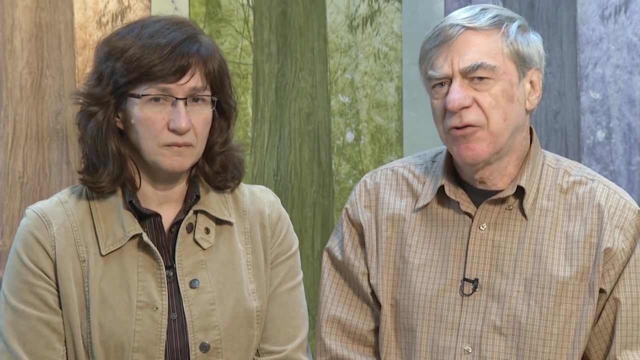 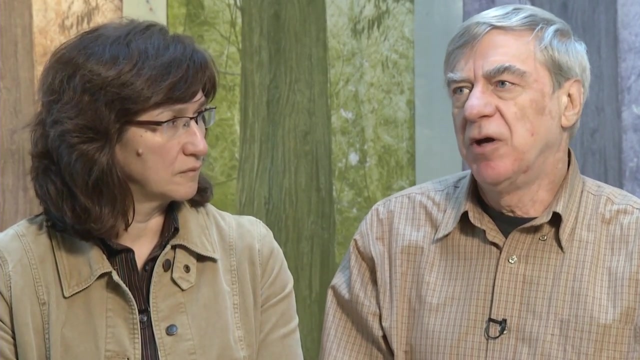 And food security, and loss of land and quality of water and so on, But general public might not be aware of these roles that soils play. I think soil science offers us some concepts around how soils form that also give us a good understanding of how ecosystems function And so. 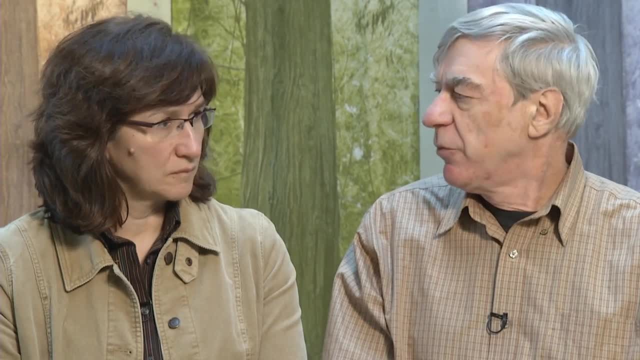 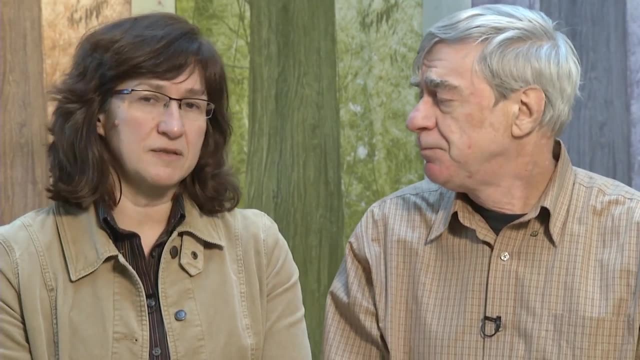 this website gives a lot of information on the soil forming factors. Do you want to discuss that? just a bit, Because that's what people are going to see on the site here. That's right, yeah, Especially if they go under the content tag that says soil classification. 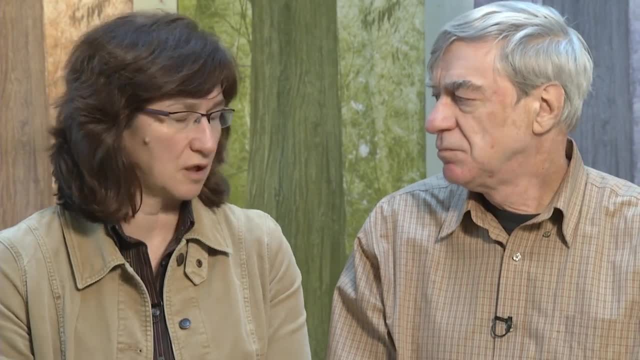 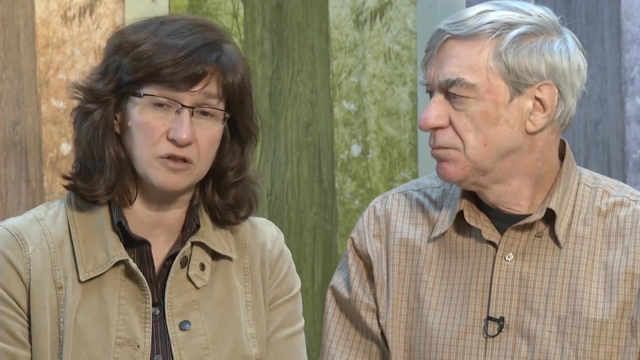 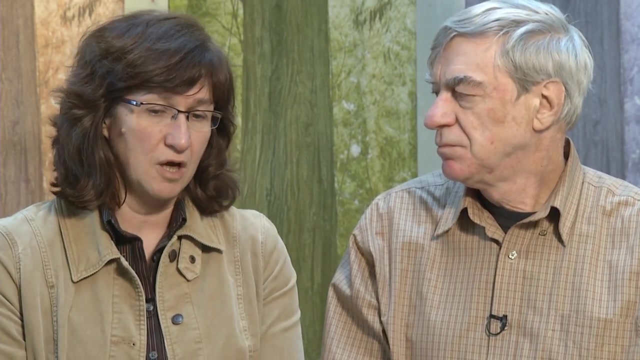 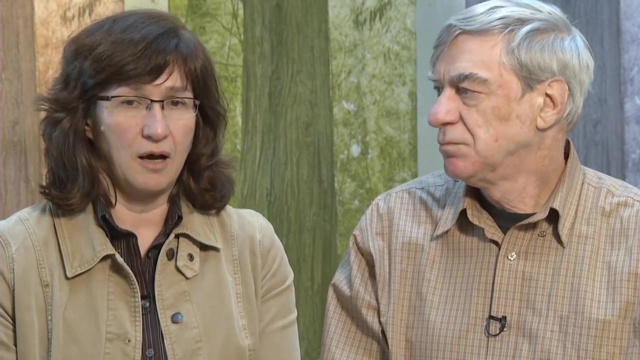 they will find several of the learning resources that talk about soil formation and various more specific processes of soil formation and soil classification. But I also hope that that kind of material will be also useful for students and teachers and general public who are interested in ecology and natural resources, because it really puts soils in the broader. 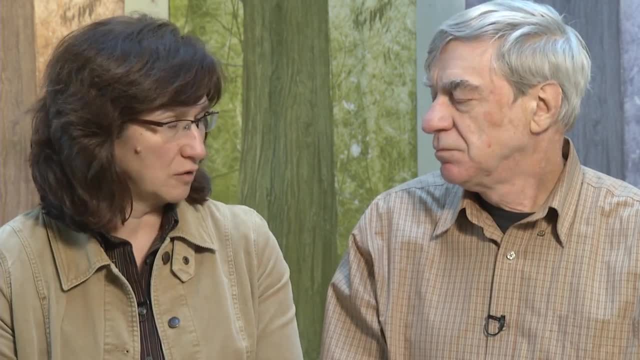 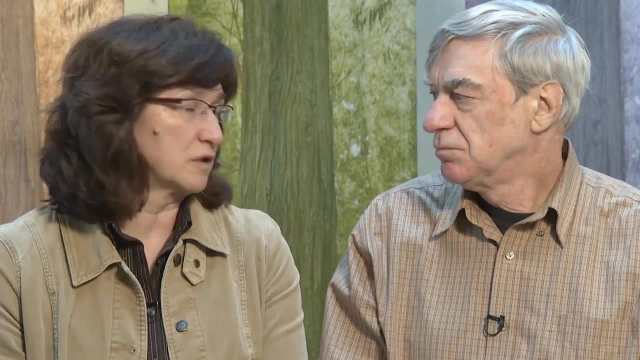 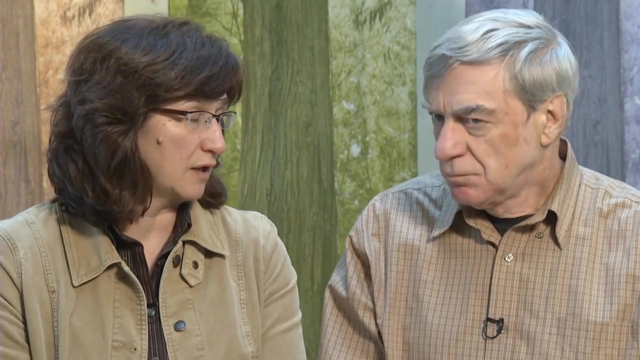 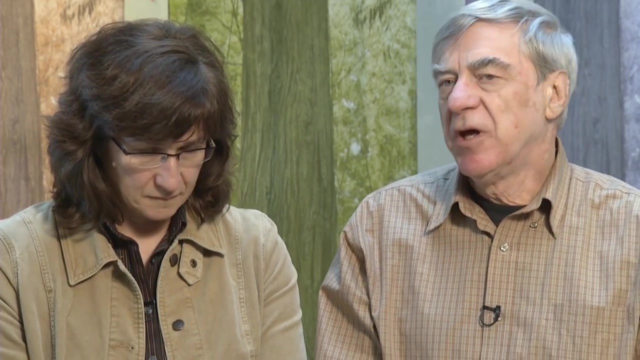 context of the environment And what are the roles that soil plays in a specific place, like grasslands of BC or northern soils in polar regions, or maybe some tropical soils in some other parts beyond Canada. So there's a lot of information here that can be taken on board to improve our knowledge. 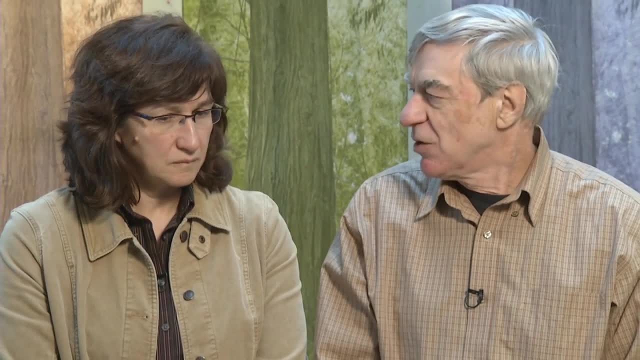 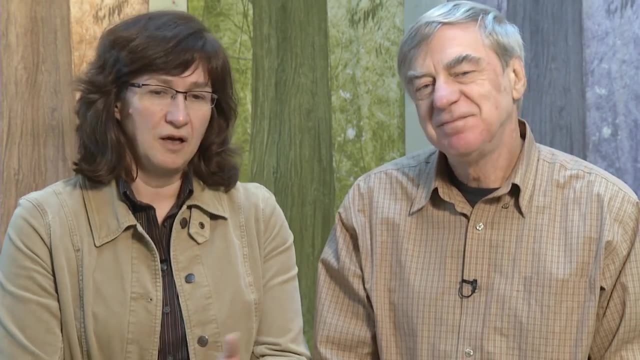 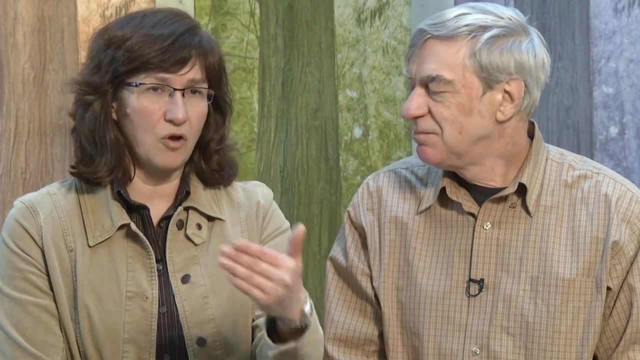 but do you anticipate any other impacts on people as they learn more about the soil resource? That's a good question, Art. I would like to believe that these resources that we developed and that we are currently working on will have a longer lasting impact on our students, and 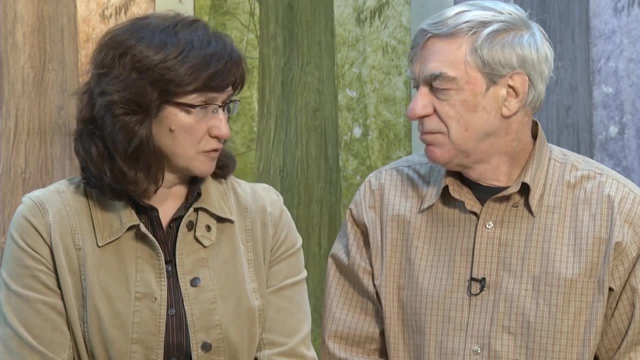 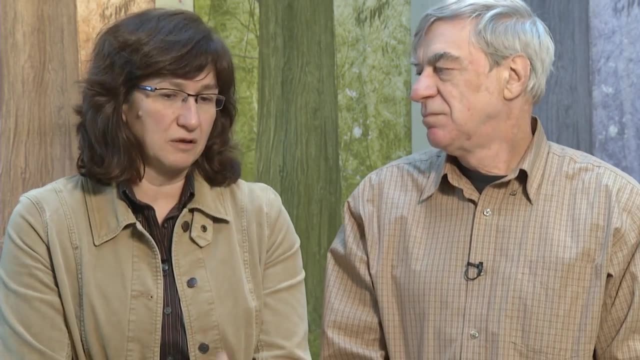 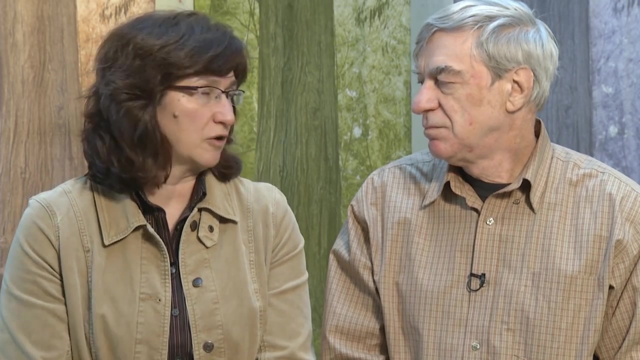 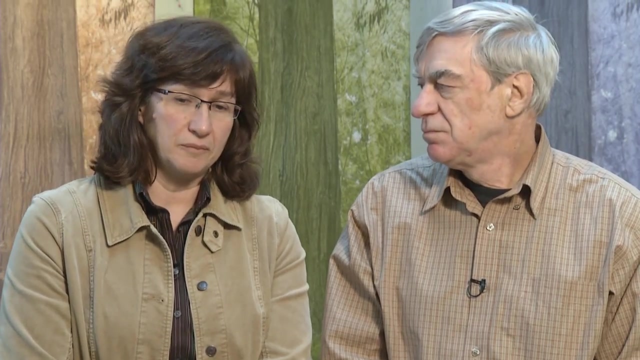 beyond, because by learning about the importance of soil and what are the roles that soil plays, hopefully everybody will understand why it's important to conserve and protect this resource, which is an integral part of the environment, and that will hopefully help somebody to further action to conserve and enhance this resource and environment in which we. 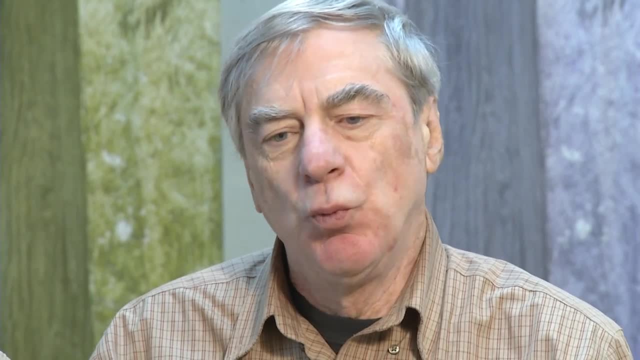 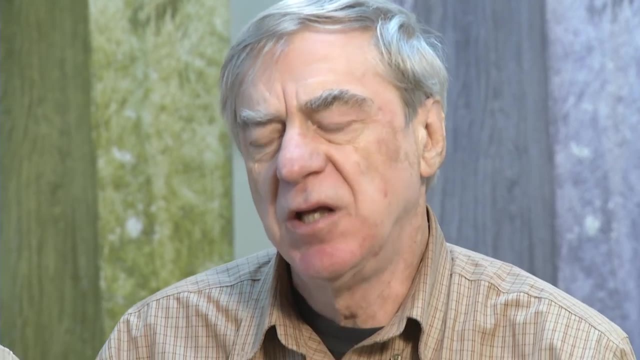 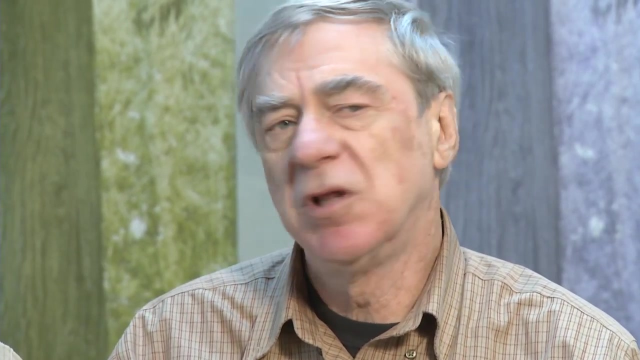 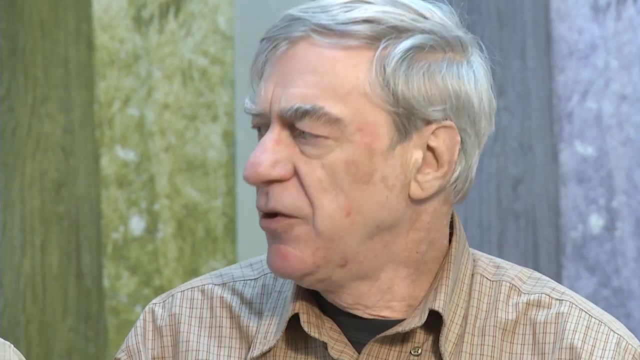 live. To sum up, then, we feel strongly that soil science is important for people to understand their environment, And it doesn't really matter whether you're interested in agricultural, forested or natural landscapes. It still offers us a unifying way to look at how these systems function. And even if you're in an